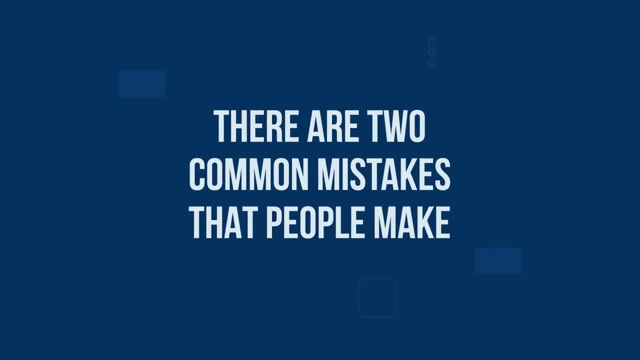 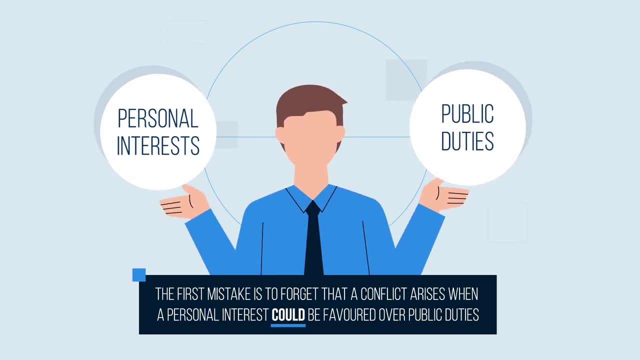 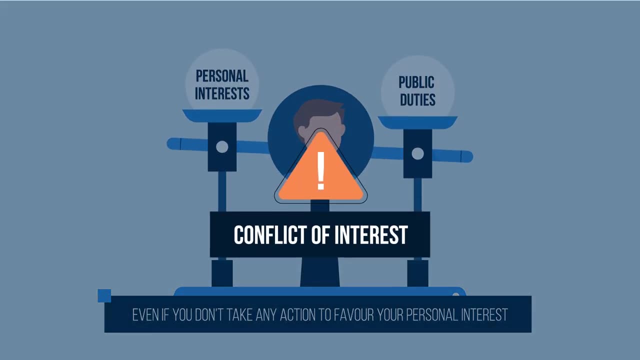 There are two common mistakes that people make. The first mistake is to forget that a conflict arises when a personal interest could be favoured over public duties. Even if you don't take any action to favour your personal interest, you still have a conflict of interest. 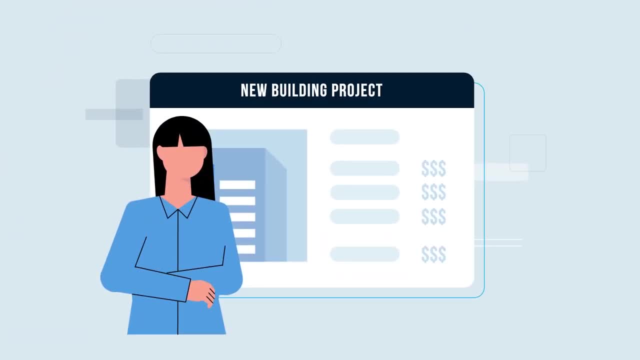 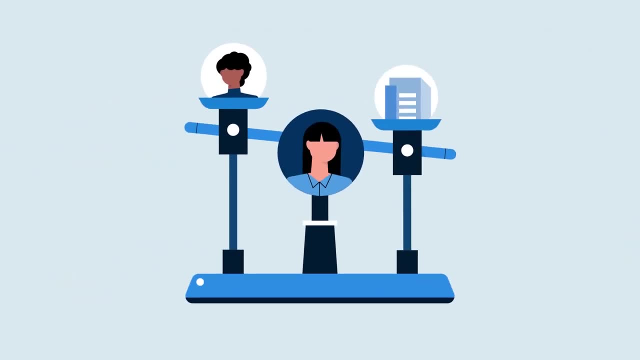 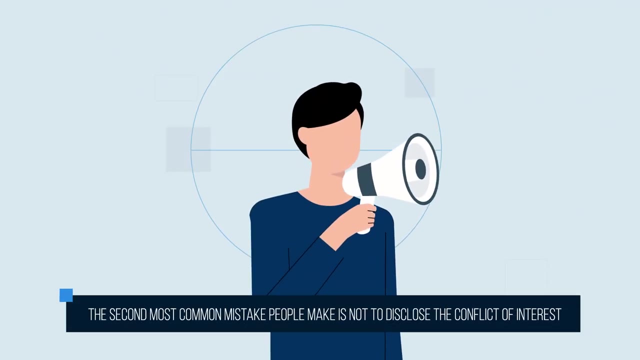 Let's take an earlier example. If a public official is working on a tender at a university and knows that her friend wants to submit a bid, She has a conflict of interest, even if she never does anything to benefit her friend. The second most common mistake people make is not to disclose the conflict of interest. 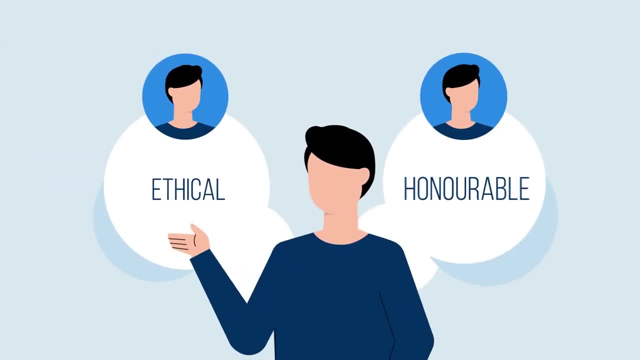 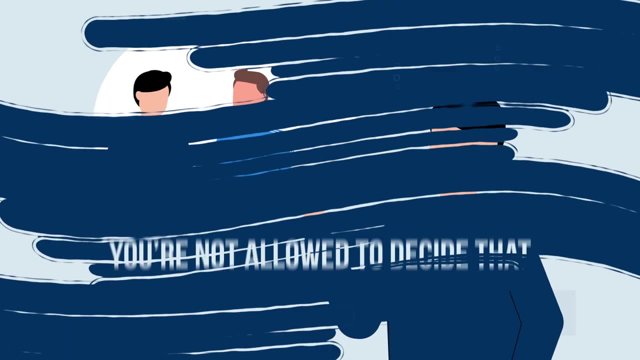 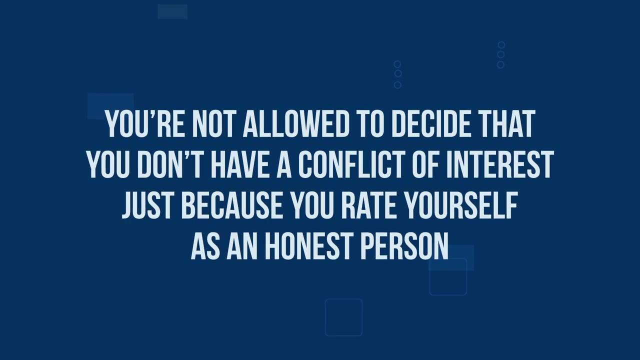 Because we see ourselves as ethical, honourable people, it can be challenging to imagine ourselves ever doing the wrong thing. Putting it another way, you're not allowed to decide that you don't have a conflict of interest just because you rate yourself as an honest person. 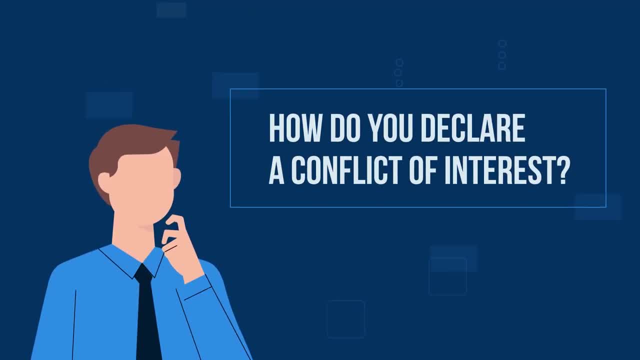 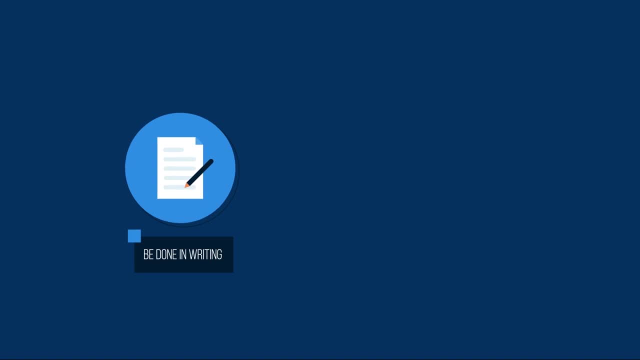 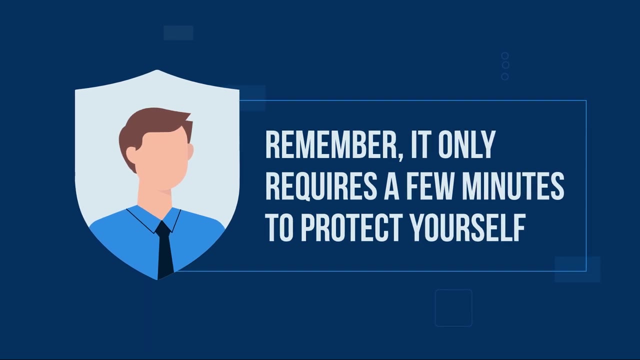 So how do you declare a conflict of interest? First, your agency should have a process in place, But, in a nutshell, it should be done in writing, be timely, be accurate. Remember it only requires a few minutes to protect yourself. 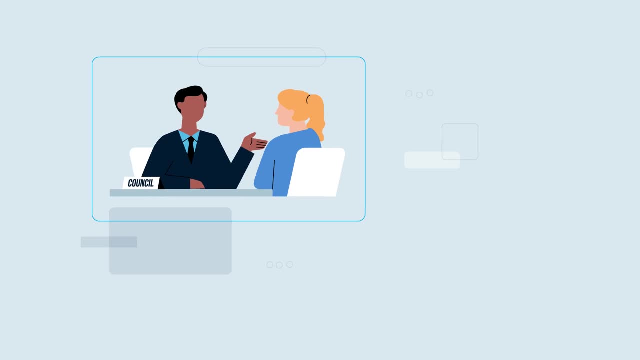 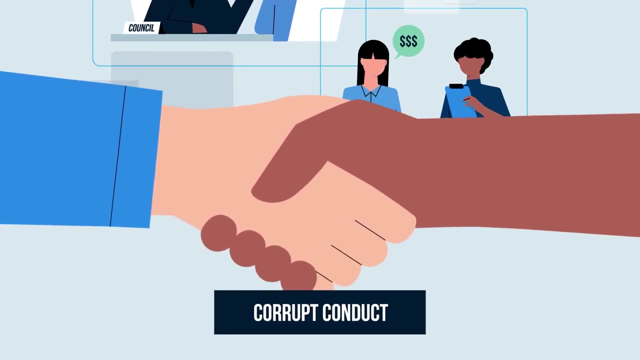 After all, a public official who takes advantage of a conflict of interest to obtain a benefit for themselves or someone close to them is probably engaging in corrupt conduct. Also, keep in mind that intentionally concealing a conflict of interest is not a good thing. 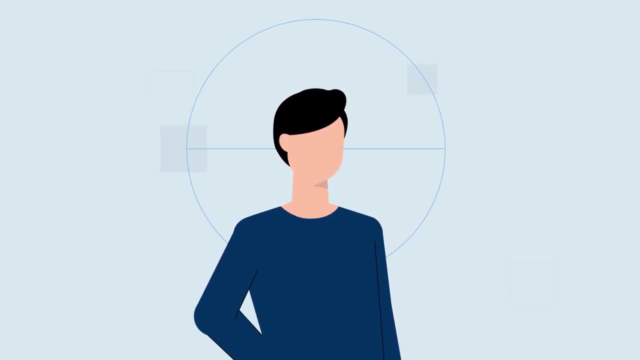 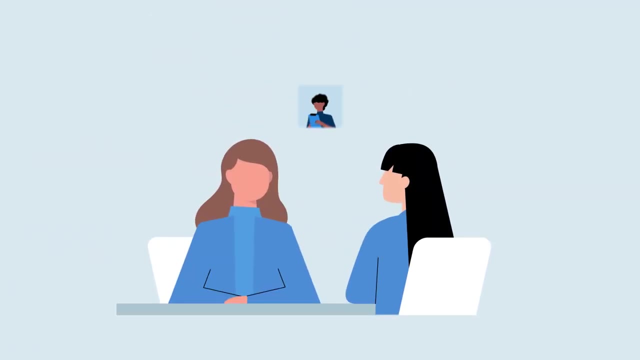 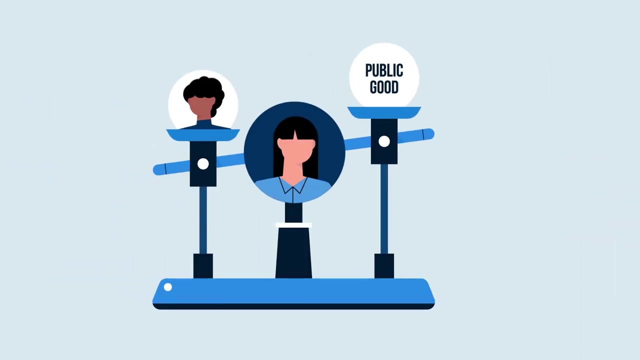 Concealing or understating a conflict of interest is dishonest and is likely to constitute corrupt conduct. Once you disclose the conflict of interest, your agency then comes up with a plan to manage it. Whatever is decided, you're expected to co-operate to make sure the public interest is put first. 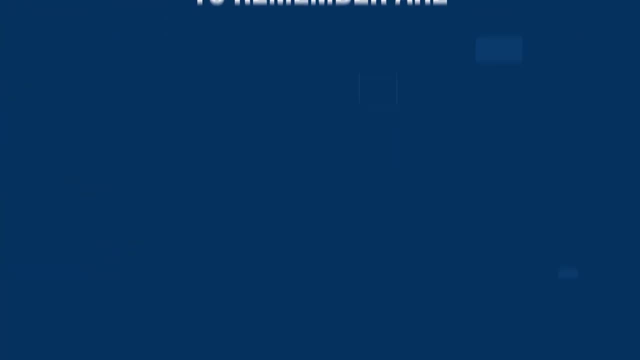 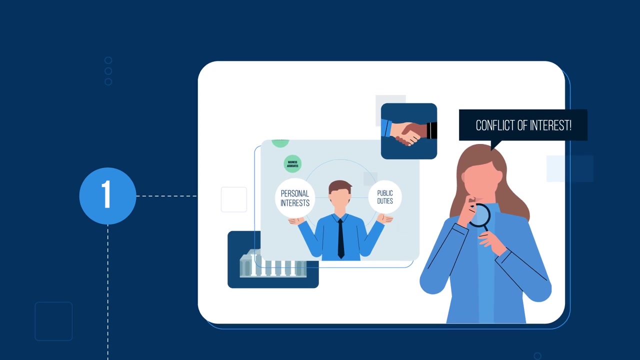 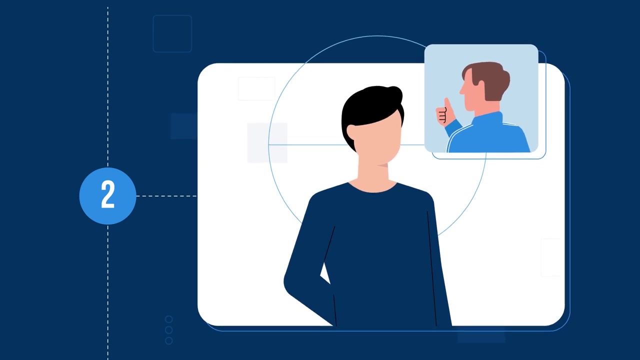 So the key things to remember are: 1. Conflicts of interest occur when a reasonable person might perceive that your personal interests could be favoured over your public duties. 2. If you conceal, understate or take advantage of a conflict of interest, you might be engaging in corrupt conduct. 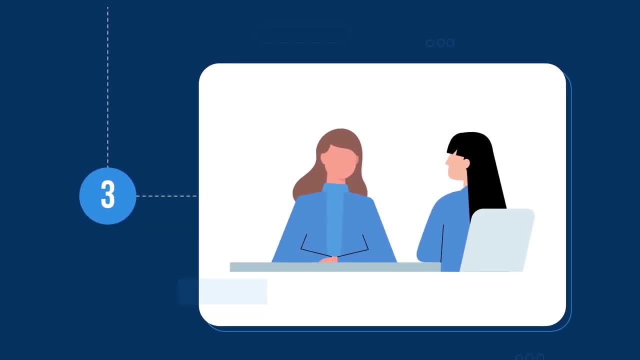 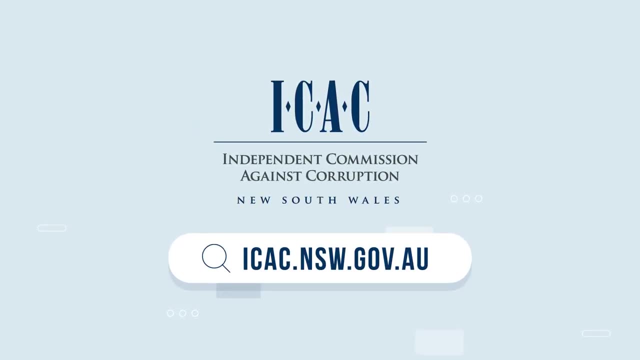 3. Disclose your conflict of interest and comply with the plan put in place to manage it. For more information, visit icacnswgovau.